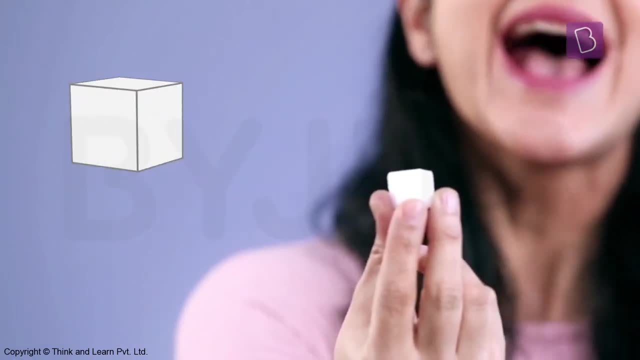 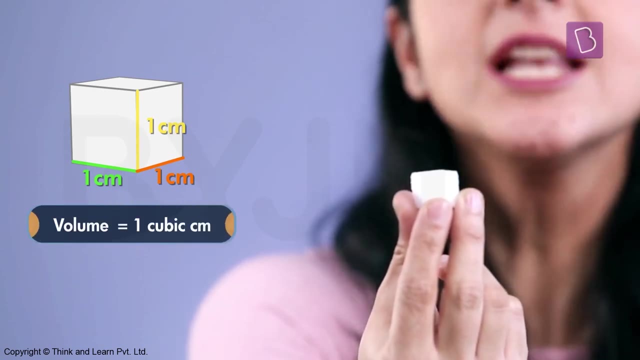 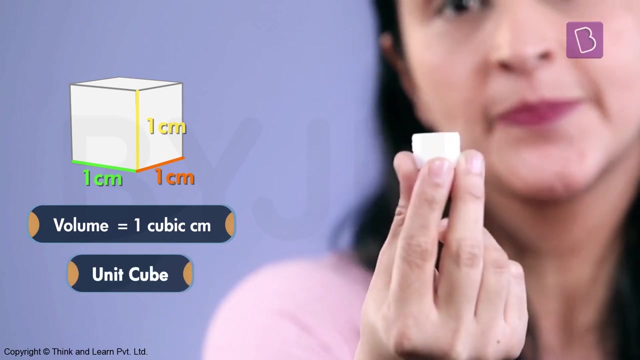 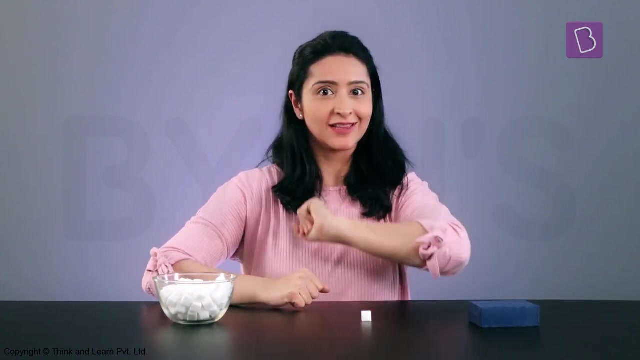 You see the sugar cube. Now, this sugar cube has a side of 1 centimetre each. This is why it has a volume of 1 cubic centimetre. That means that each of these are unit cubes. Hey, I can now build a cuboid using these sugar cubes. Let's do it. 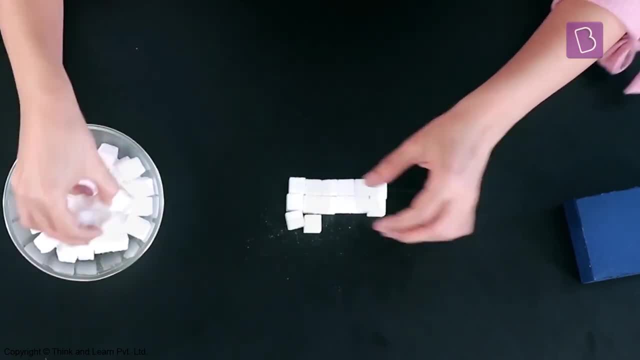 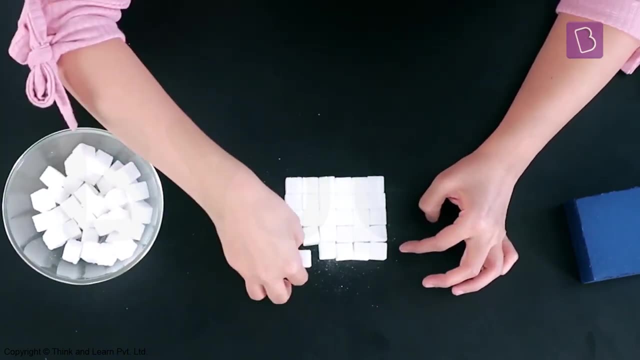 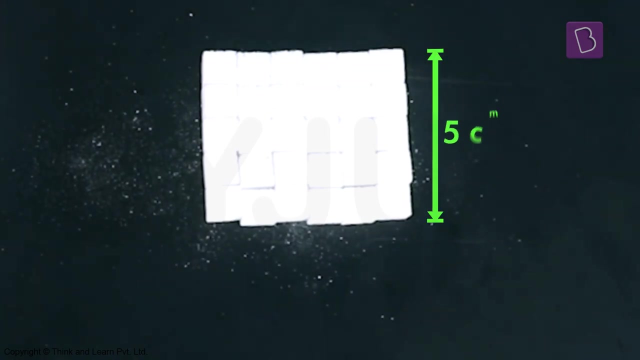 All right Now. this cuboid has a length of 5 centimetres because I put 5 sugar cubes this way. Similarly, the cuboid has a width of 6 centimetres Because I put 6 cubes this way. So how many cubes did we use here? 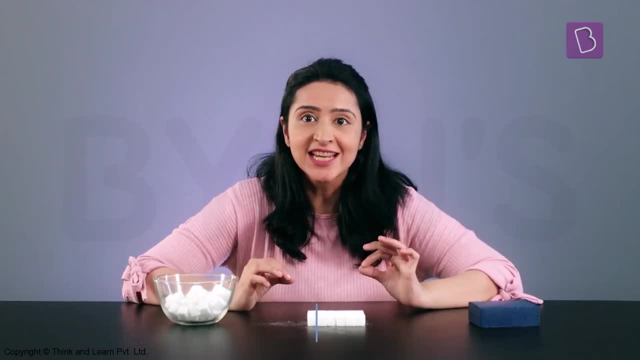 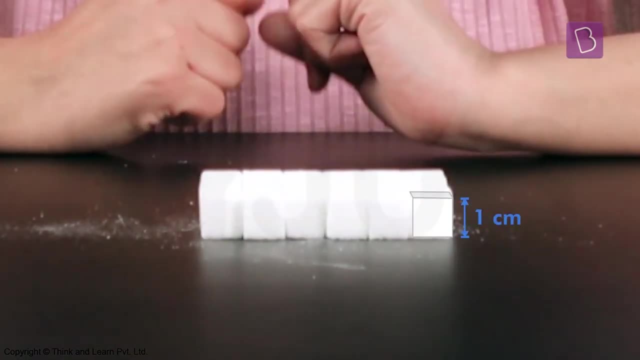 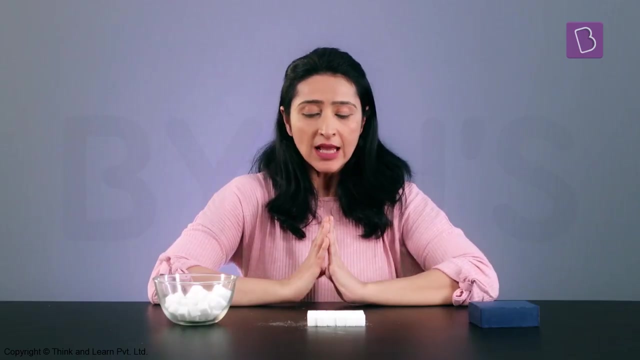 30, right. Another way of writing is 5 times 6.. But this is just 1 centimetre tall. Why? Because each cube is 1 centimetre in height. Now, this means that if I have to make it larger, I have to make it Notre Dame. 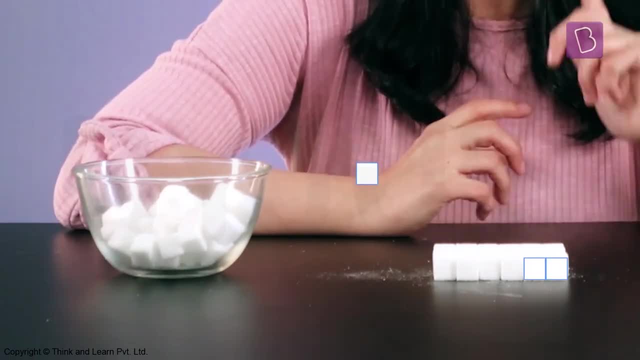 That means that if I have to make it larger, I have to make it Notre Dame. That means that if I have to make it larger, I have to make it Notre Dame 2 centimetres tall. I will need one more layer of these cubes, So let's do it. 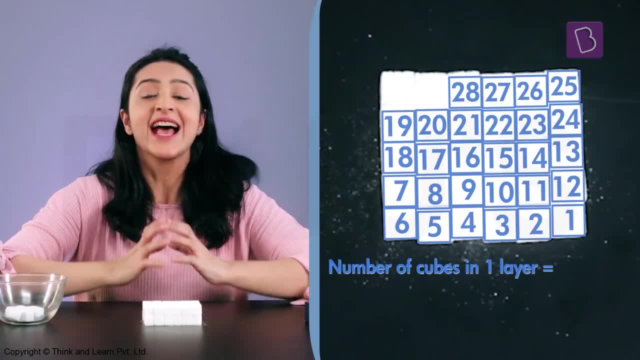 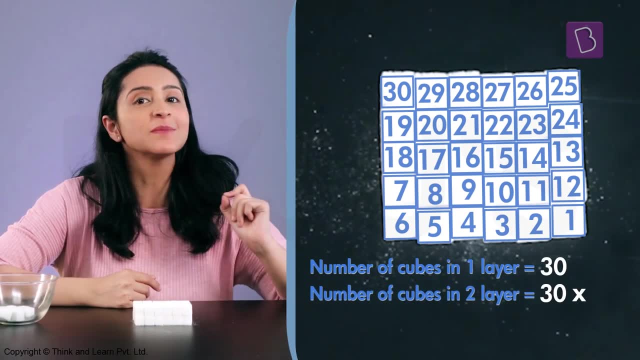 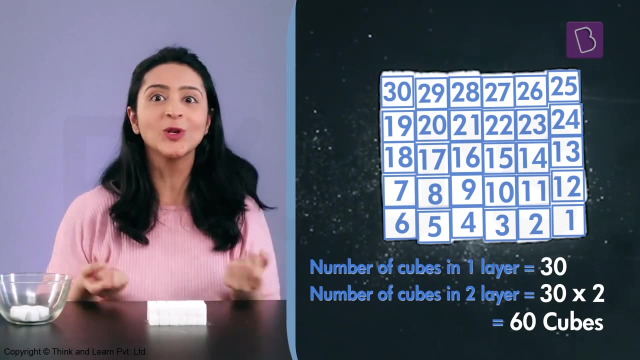 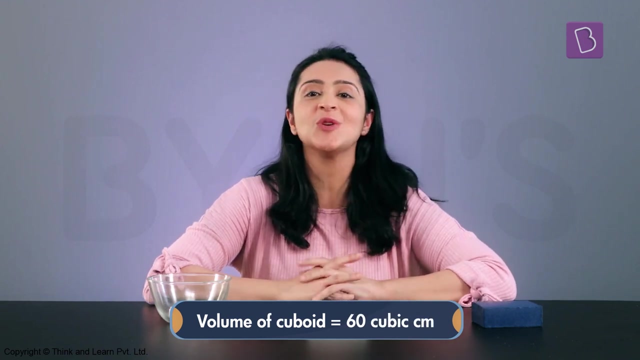 Voila Now. if one layer has 30 unit sugar cubes, then two layers will have 30 times 2, which is 60 sugar cubes. And this is nothing but the volume of the cuboid. So the volume of the box would be 60 cubic centimetres. As I said earlier, volume is the. 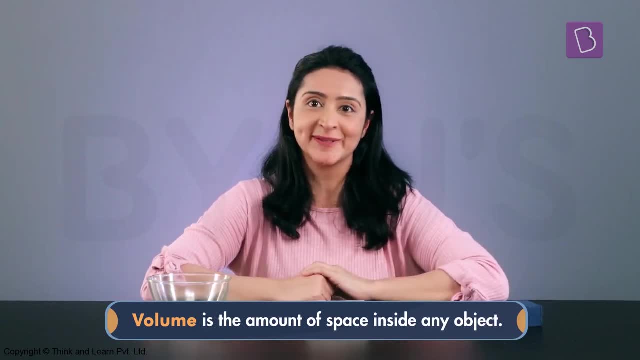 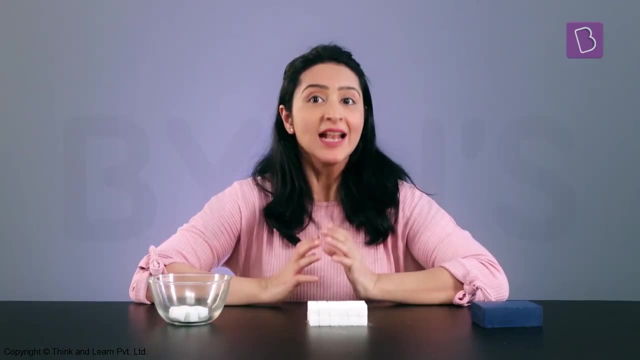 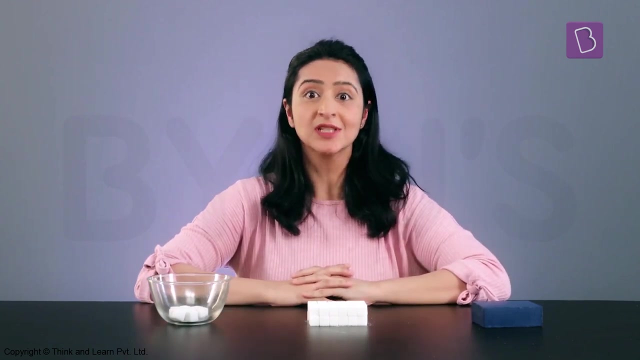 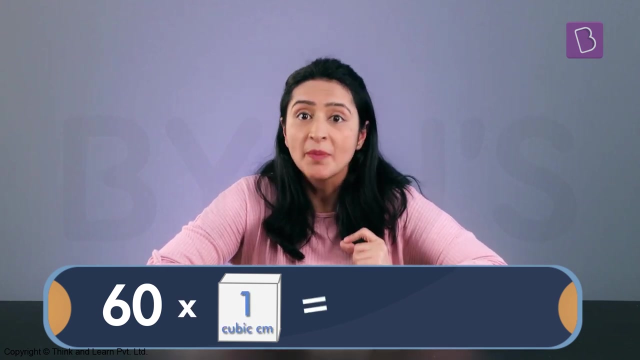 amount of space inside any object. What we did here was fill up this space with unit sugar cubes. Now to find the volume, all we have to do is just count the unit sugar cubes, So 60 cubes of 1 cubic centimetre each to make up a volume of 60 cubic centimetres.